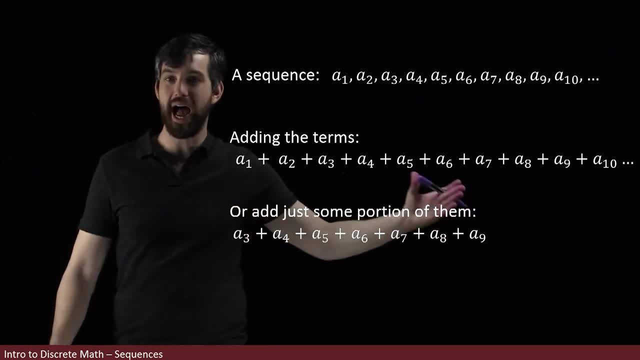 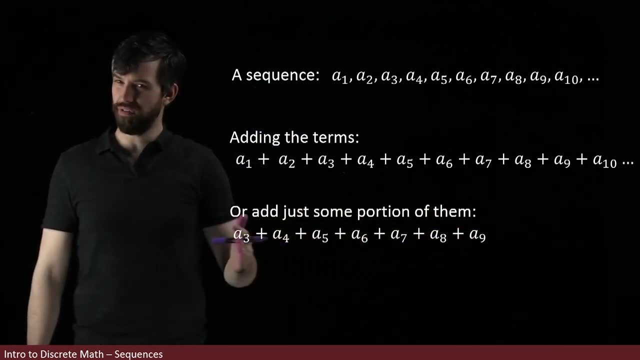 but I want to take a3 plus a4, all the way up to adding up a9.. And that's the group that I want to sum up. Well, this thing here is if all of these are integers, just going to be some other integer. 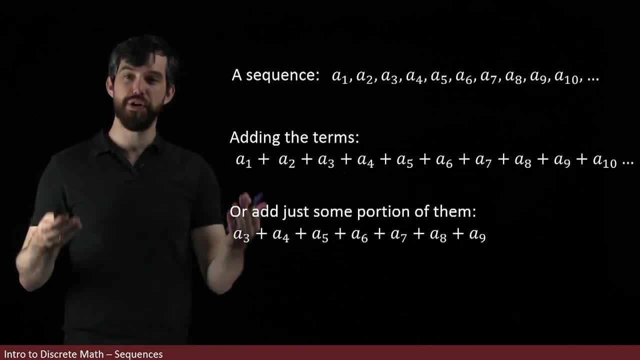 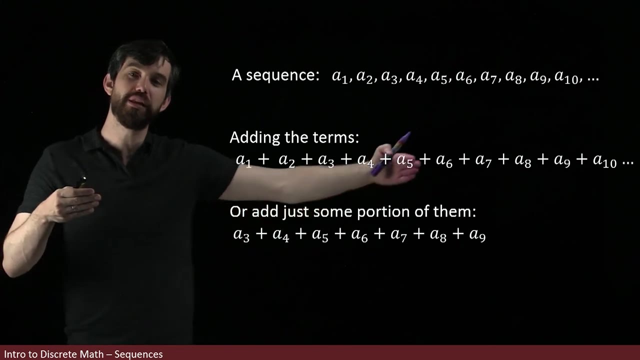 Now we have a formalism, a new set of notation, because I don't want to have to write all of these down, and I chose a9 mainly because I was getting bored typing, But in an actual problem, maybe a9 here is supposed to be a million and that you've got this really, really large number of things that you're adding up. 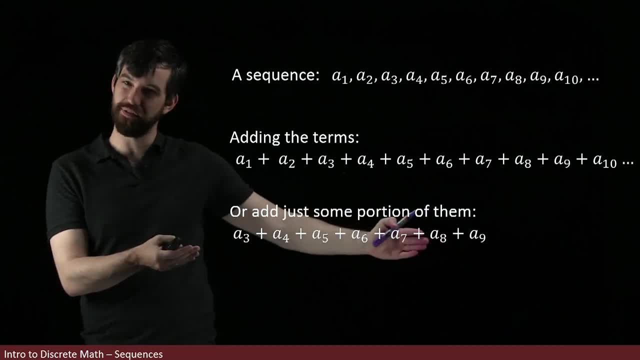 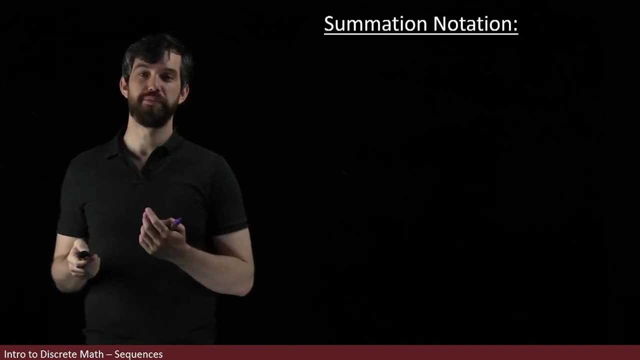 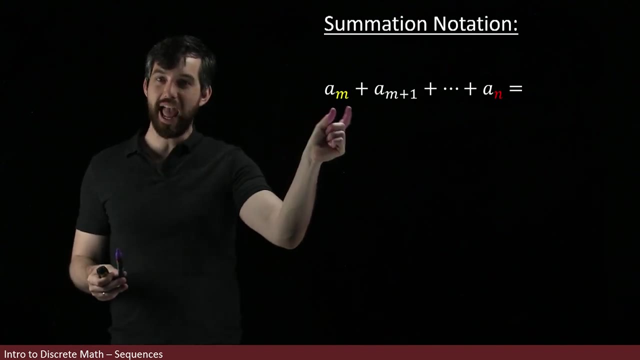 So I want some notation that can express this very long list of things in a really nice short way. So the way I'm going to do that is something called summation notation, And what we're going to begin with is just some sum, And I want you to note here that I begin on an mth term. 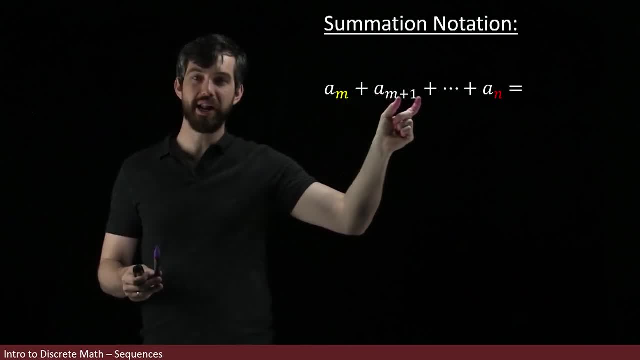 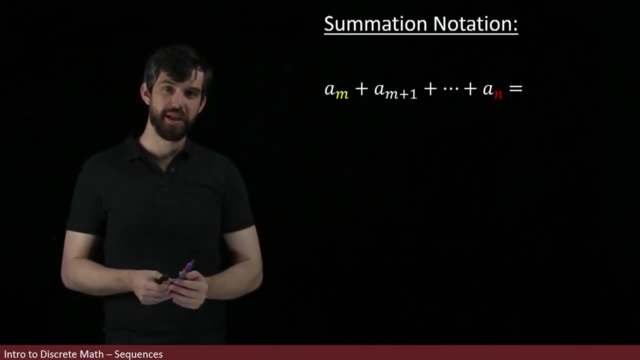 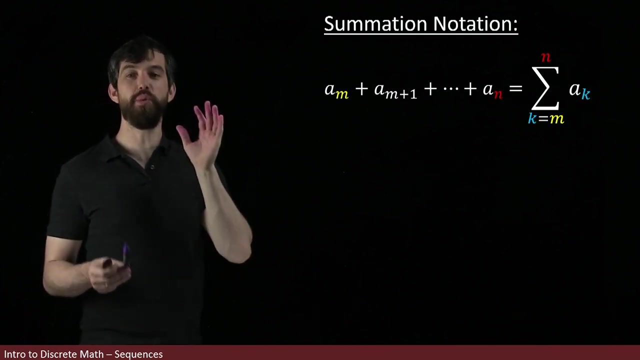 And then I go to the mth plus one, the mth plus two. I keep on adding, on, adding up, and then I end at an nth term. So I go from an nth term to an nth term And then the way I'm going to make a shorthand for this is this notation here, which looks a little bit. 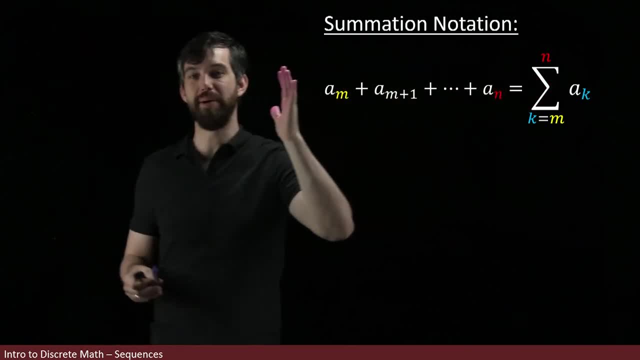 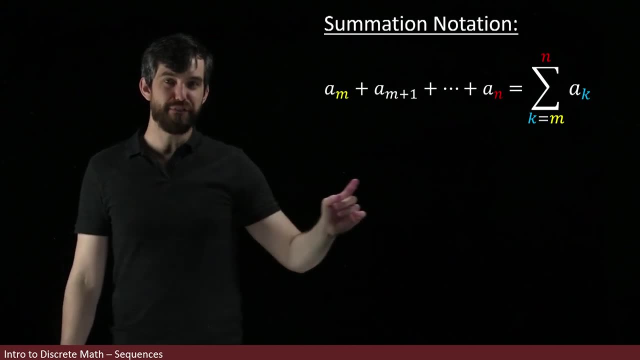 weird if you haven't seen it before, but this symbol here is called a big sigma, but I usually just say it's the sum And we have a couple different things. First of all, down on the bottom there's the m. That was my starting point here, right? So I've got the m, which is my 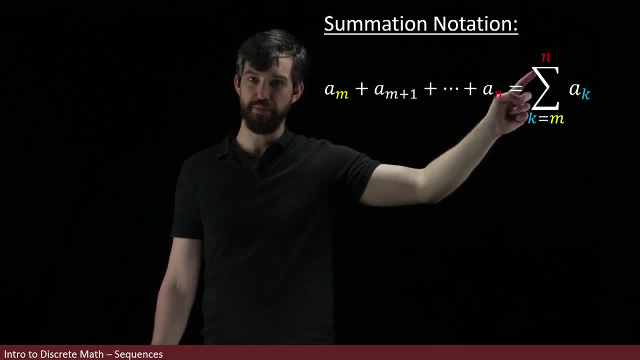 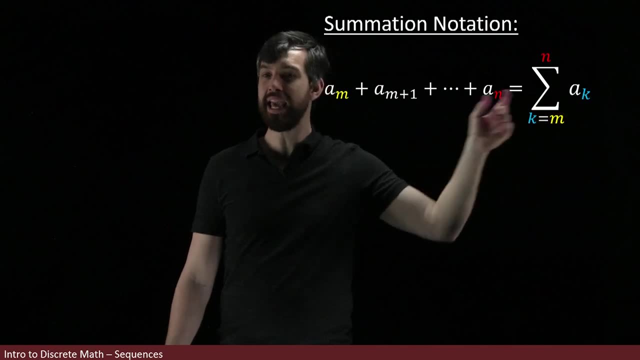 starting point And then I go up to the n, which is my finishing point. So it's like start at m, go up to n. I'm taking the sum of the a k's, where a k is like the generic kth term in my 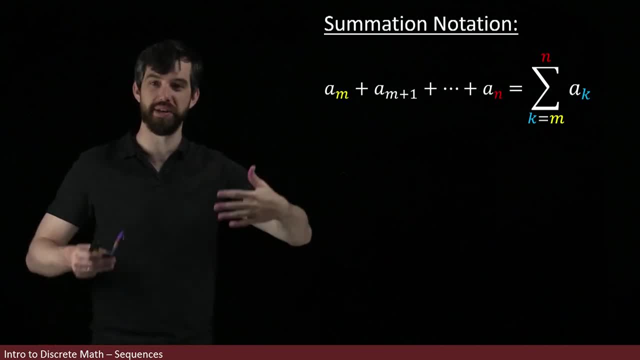 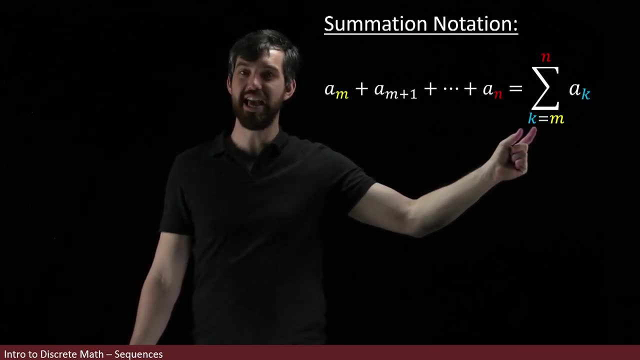 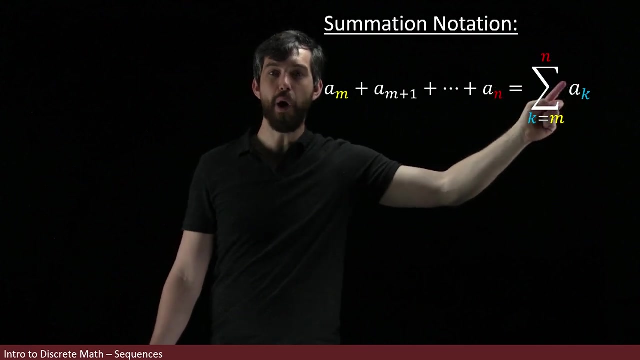 particular series that I'm summing up. I use series for sum and sequences for a list, And then the way I write it is I say that my index variable, that k, the k is the one that's changing. This is thought of as the k starts at m and goes up to n, And I'm summing up all of the a k's. 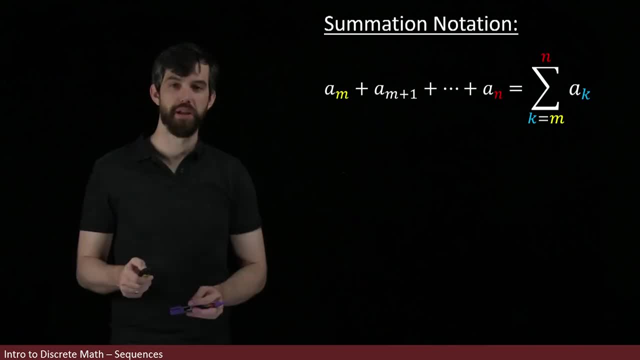 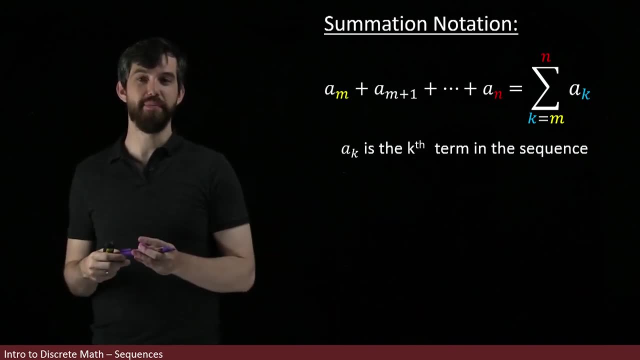 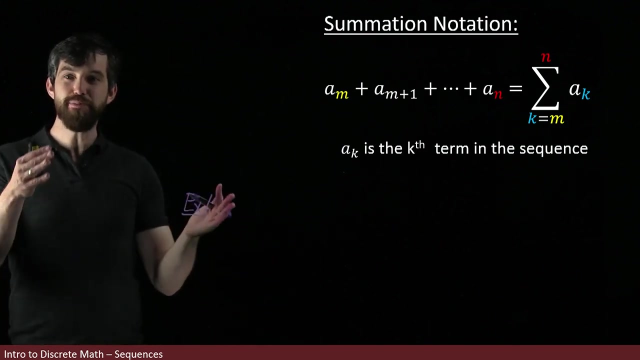 in that region from the m up to the n. So here the a k is thought of as that generic kth term in my sequence. Okay, so let's see how we might run this out in an example. I want to keep with our familiar example of a k. 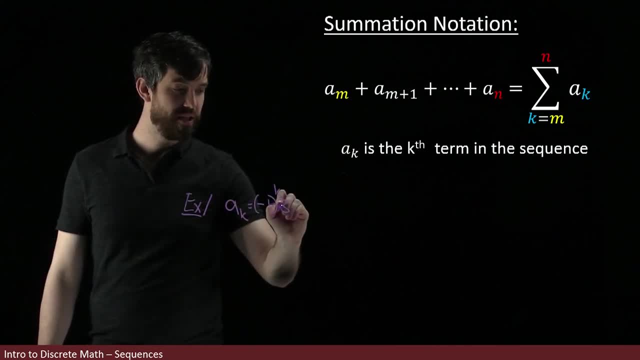 being the nth term. So I'm going to take the nth term and I'm going to take the a k and I'm going to the minus one, to the k, three k, And then what I'm going to do is- I want to try to compute this- 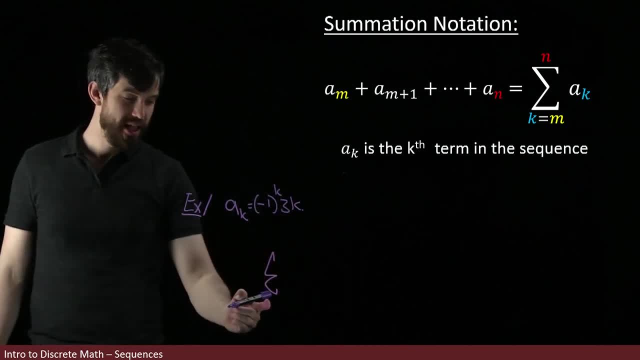 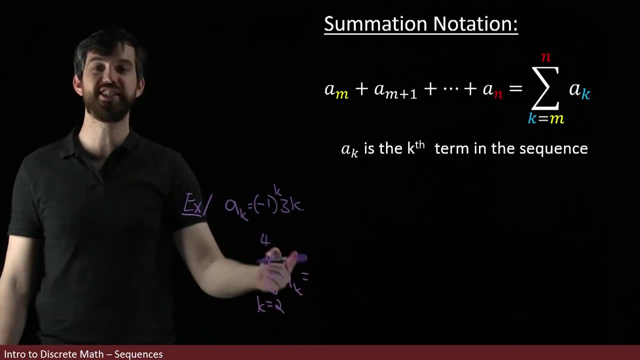 thing. I'm just making one up at random. I'm going to take the sum and I'm going to do k equal to how? about two? up to four of the a k, And I want to try to sum this thing up. Well, what we can do. 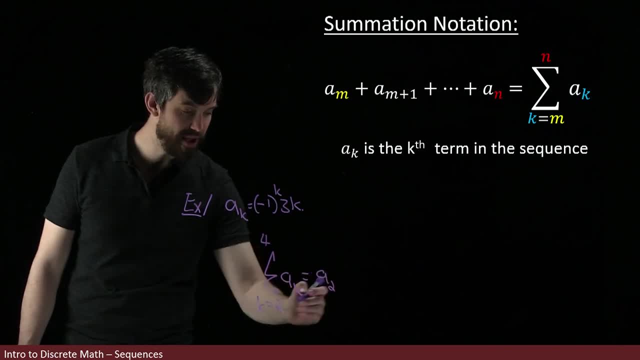 here is: okay, let's do the a two. That's my first term, starting at two. Then I add the a three And finally I'm going to go up to the a three, And then I'm going to add the a three And then I'm. 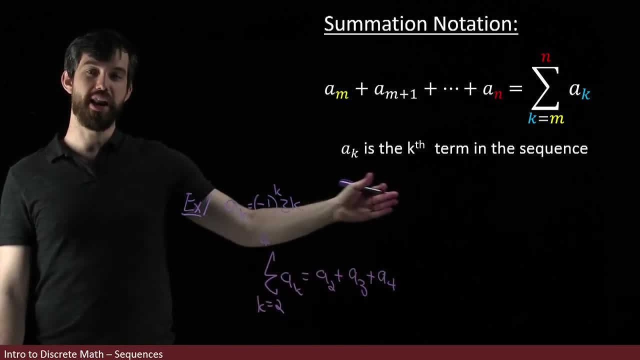 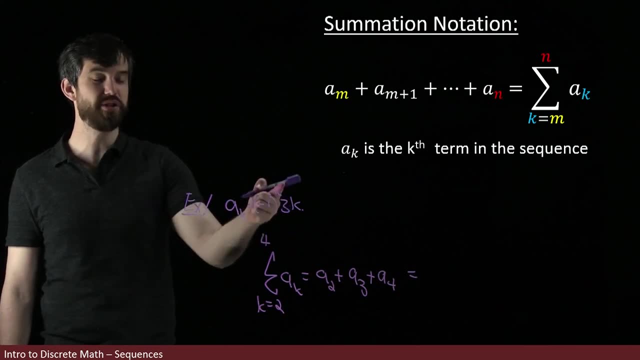 going to add the a four. So those are my terms: a two, a three and a four. And then we've seen previously what these terms were Like. if I want to do the a two, that's k equal to two, So minus. 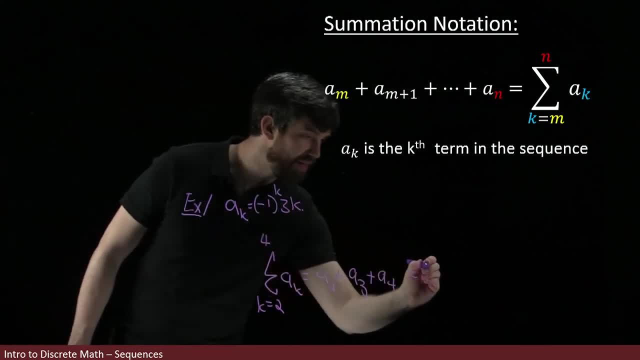 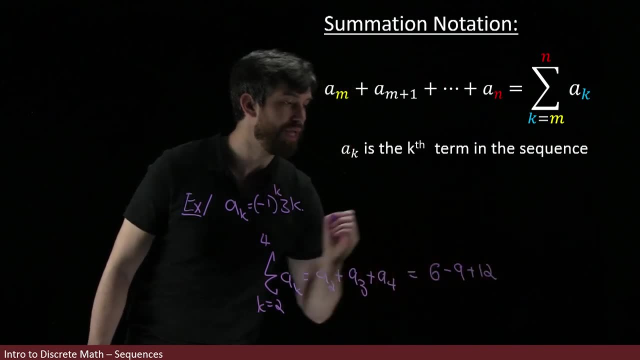 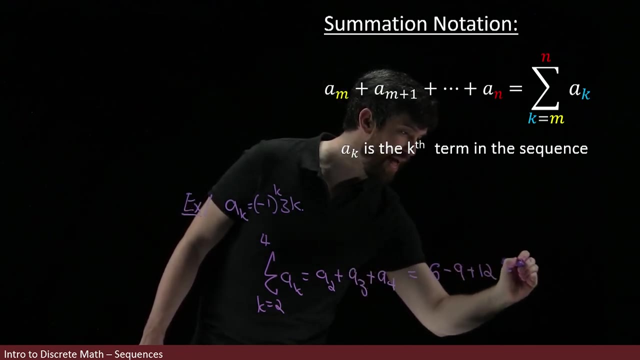 one squared, it's going to be a plus one three times two. So this is going to be six, And then the next term is minus nine And then the next term after that is going to be plus 12.. And this looks like six and 12 is 18 minus a nine. This looks like it's going to have the value of nine. 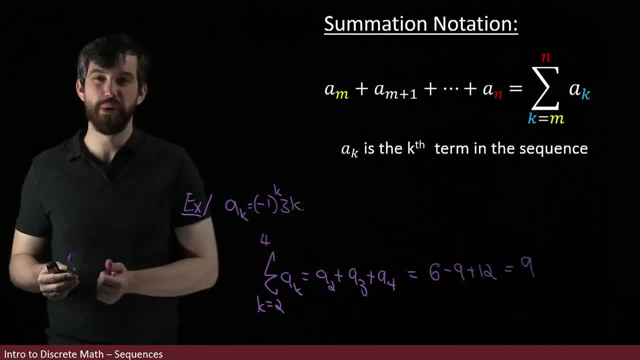 So, in other words, there's a lot of fancy notation to do a sum with only three things. The point is to deal with ones that are much more than three, But we can see this in the simple example: the sum from two to four of this particular sequence is going to be this expression, And we can add them. 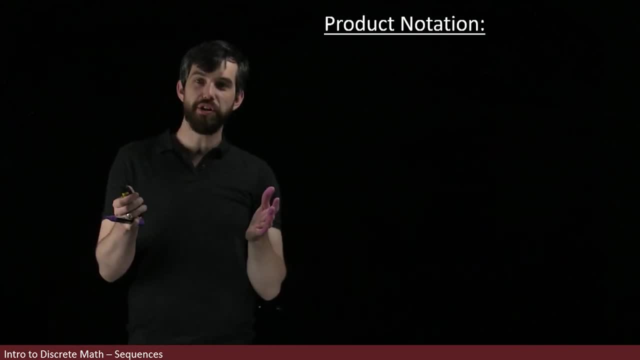 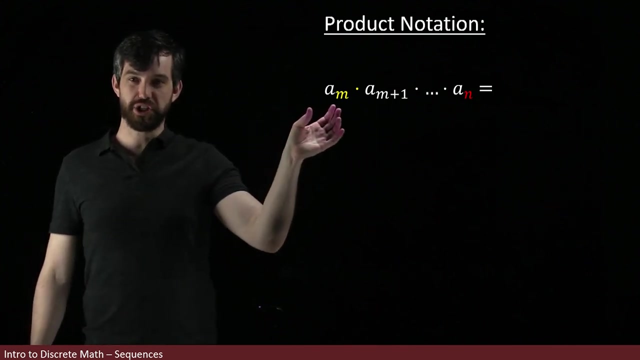 up and it gets to the value of nine. We can do much the same thing with products. For example, if I have some sequence, I could be interested in multiplying together a bunch of consecutive terms in my sequence. So, for instance, suppose I wanted to start at the mth one and I wanted to end. 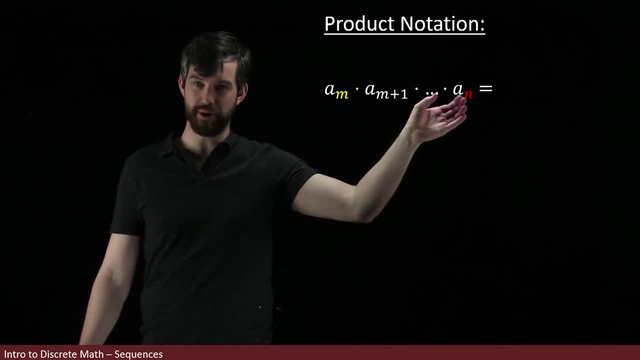 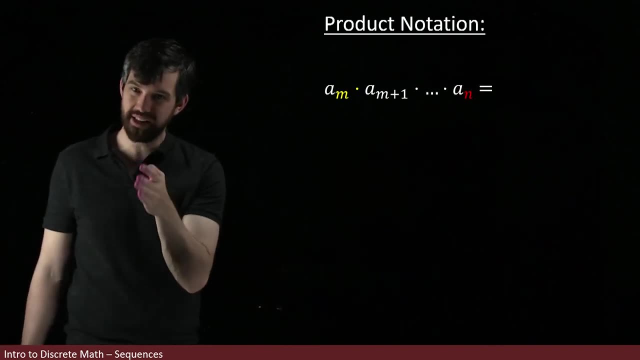 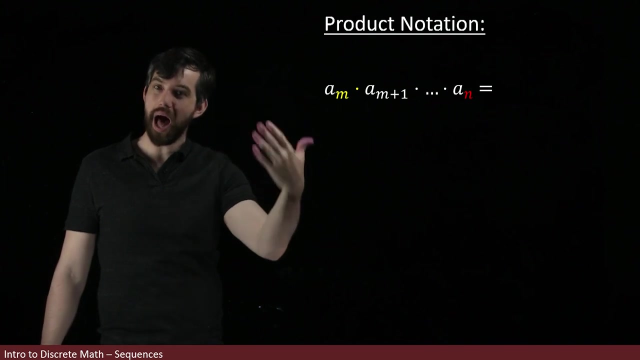 at the nth one, I could just say: what's this product of all the sequential terms between m and n? And then my fancy notation. my product notation for this is almost exactly the same thing, But where before I used a capital sigma to denote sum, here I'm going to use a capital pi. 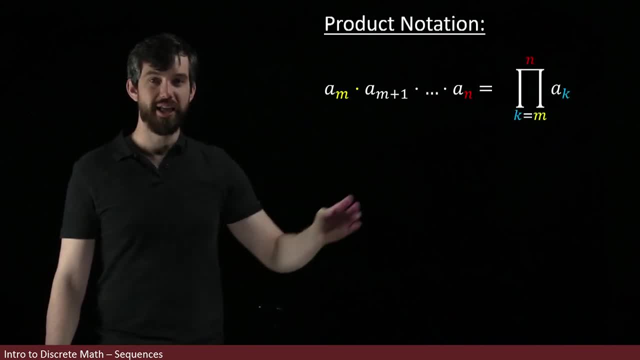 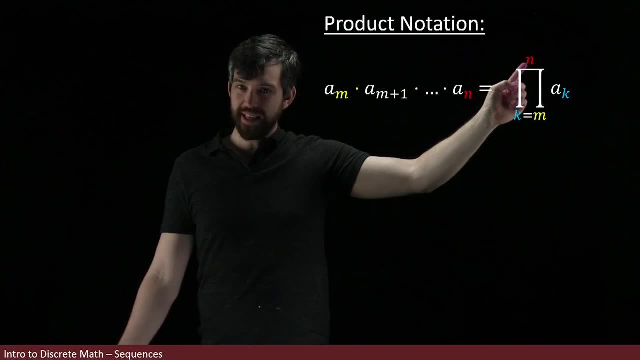 to denote product. So this is my notation. It's a pi symbol, but when I write it in this way I just say it's the product, Where I start at the m and I end at the n and I'm taking this product of all the generic a k's where that k ranges between the m. 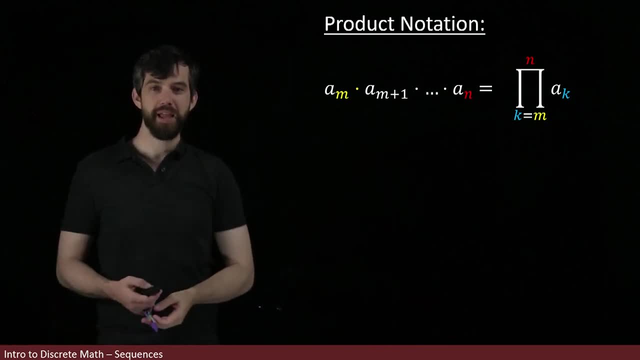 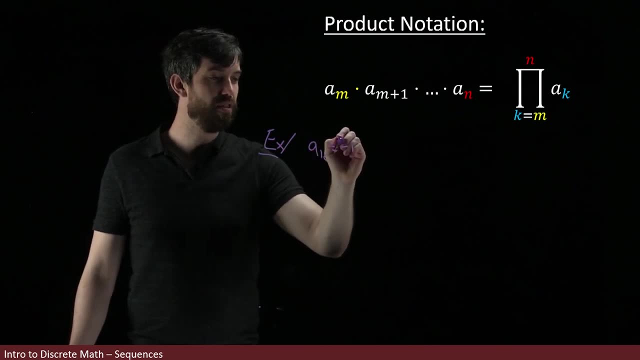 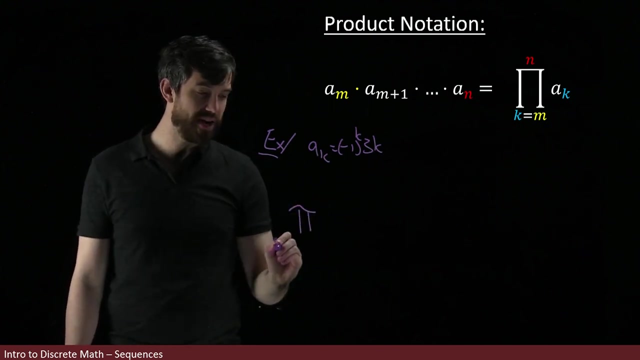 and the n. So that's my notation here, And I can likewise take that same example that we've been doing a few times now: the a k equal to the minus one to the k times three k. And I could take now, this time, the product. 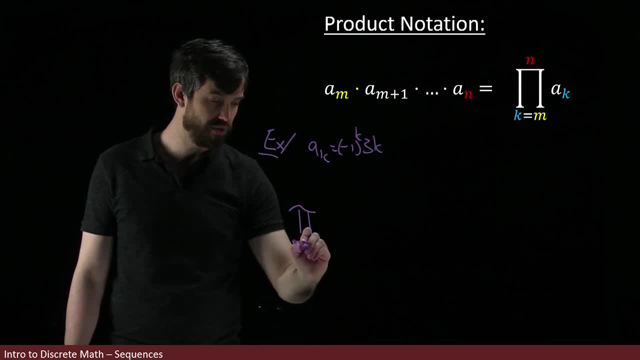 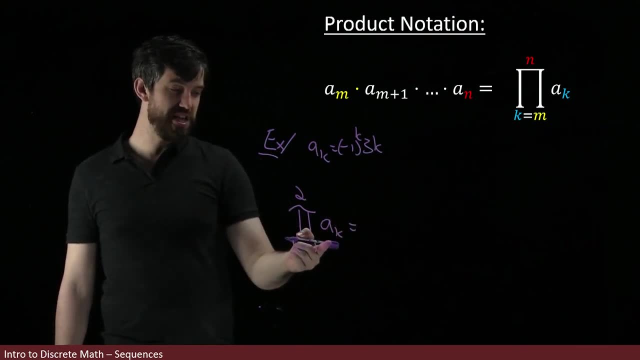 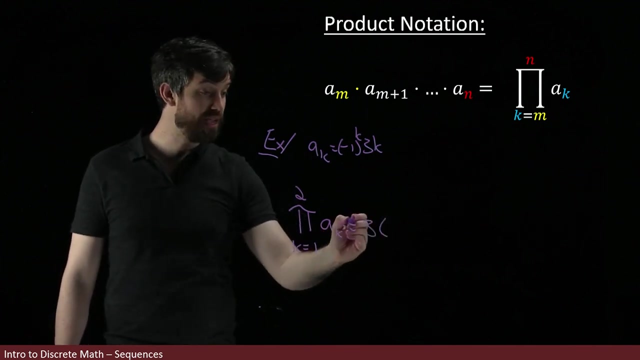 Of a bunch of different numbers. how about k equal to one, up to two? just to keep our lives simple, of a k, The first a k is going to be the value of three And the second a k, excuse me, of minus three. 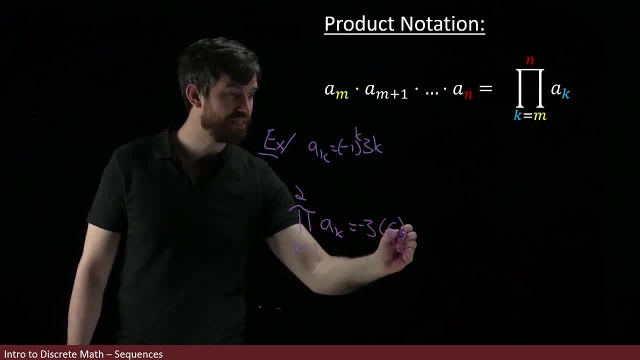 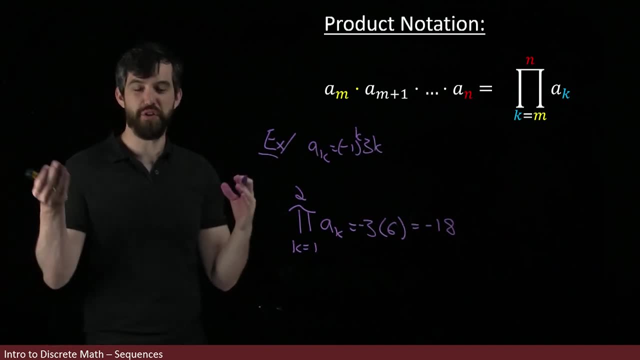 And the second a k, is going to be the value of six, And so this product is going to be equal to minus 18.. And likewise, for the most part, what we're really interested in practice is much larger product than just two terms. We wouldn't. 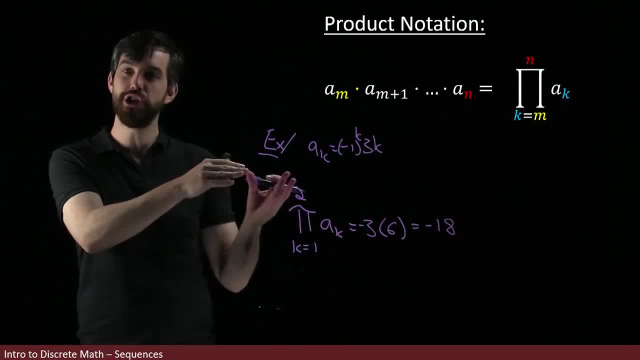 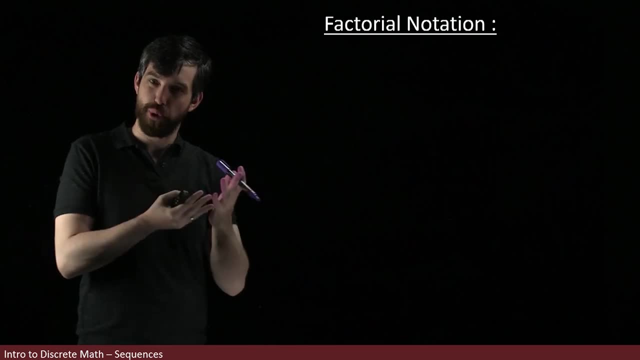 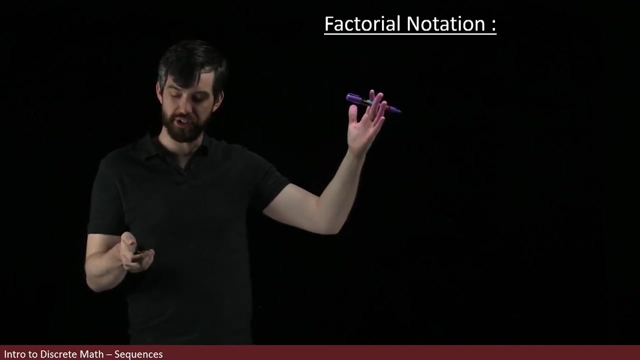 bother with notation if we only cared about two terms. But the notation generalizes to a very large number of terms. There's a special sub-case of product notation that's important enough in its own right that we actually give a whole new notation for it and call it factorial notation. And this is when I'm 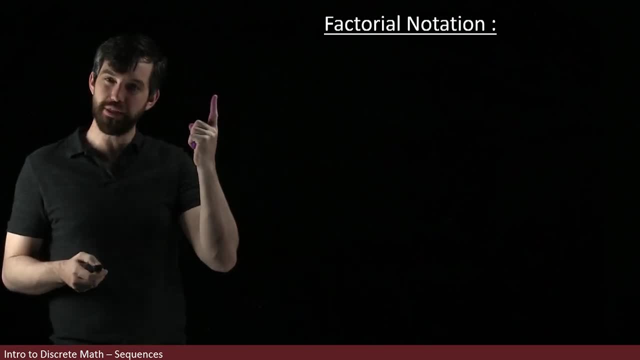 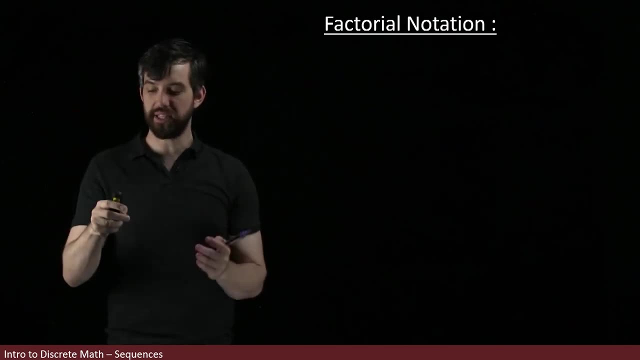 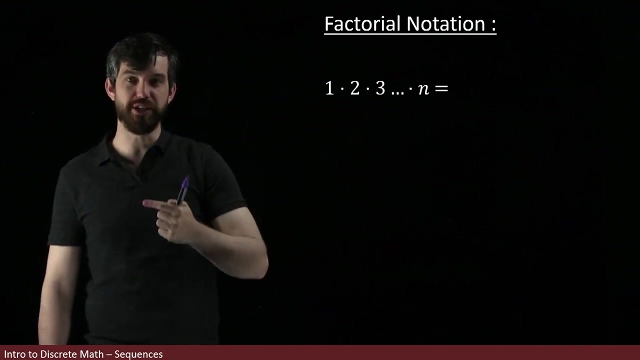 taking the product of a bunch of terms, but I'm specifically looking at the sequence a k equals k. That is that sequence: one, two, three, four and so on. That is the sequence that I want to look at, So the product of the first n terms. if I want to use my old notation, I can write it like this: 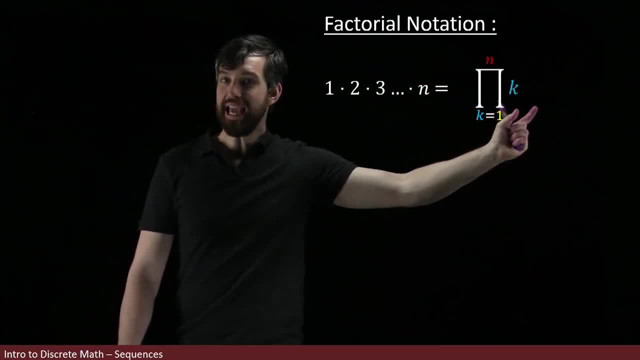 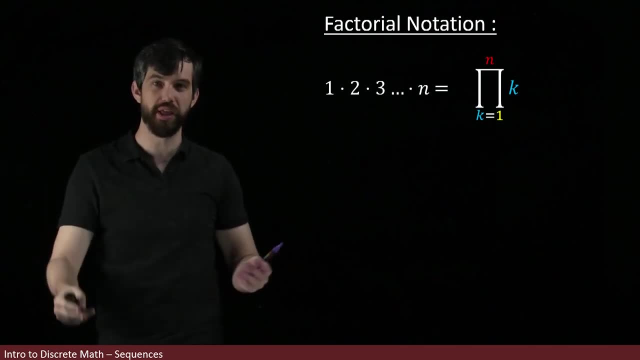 I can say that it is the product where my a k here is just a k equal to k. The first term is just one, the second term is just two, the third term is just three, So the a k here is being replaced with k. 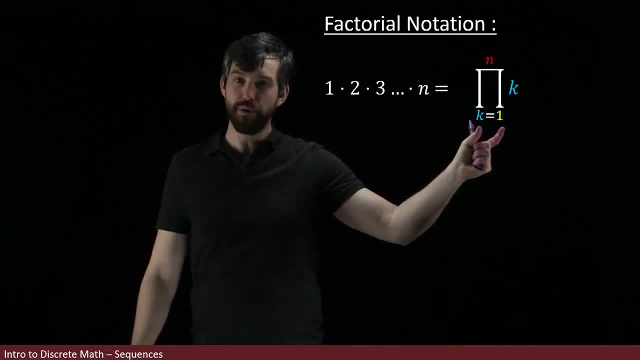 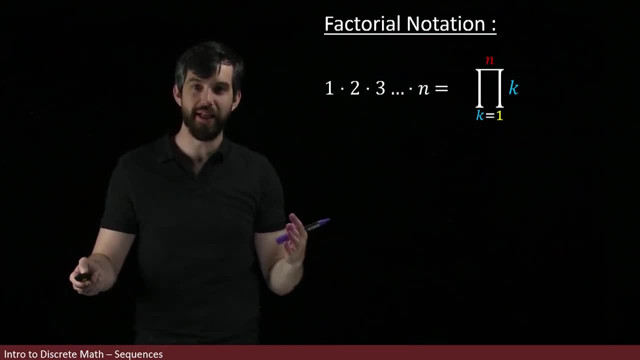 because it's a very specific sequence. And then I'm going from k equal to one up to k, So I'm going to k equal to n. This particular multiplication is defined to be factorial and the other notation for it, our shorthand for it. 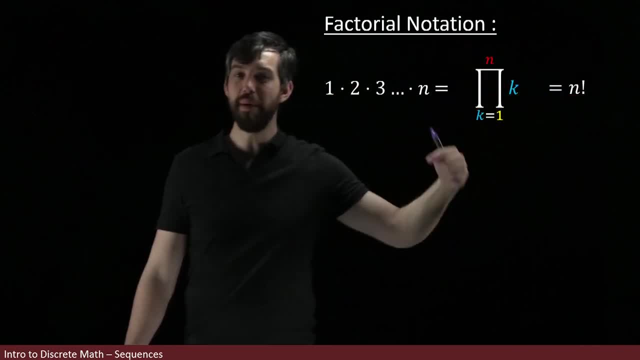 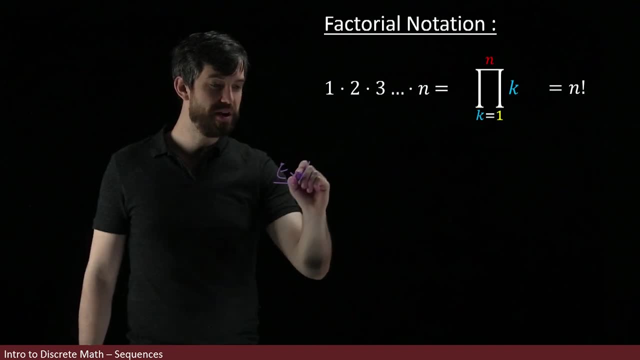 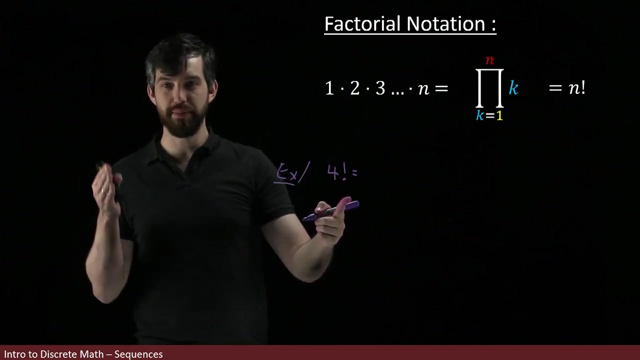 is gonna be an n, and then I put a little exclamation mark, and the exclamation mark means this particular product. So, for example, if I wanted to compute, say, four factorial, I'm gonna say that this is one times two times three times four. or if I wanna do it the other way around, 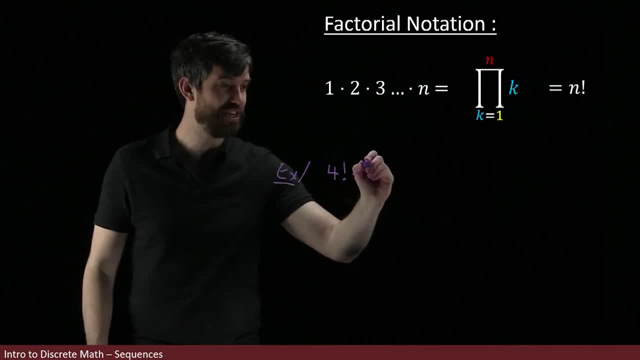 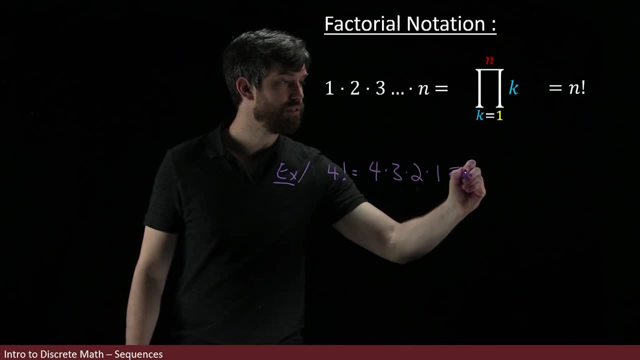 which for some reason seems to be how it's most often represented. So I'm gonna have to do it the other way around: Four times three times two times one, which is six times four, so 24.. And that is gonna be four factorial. 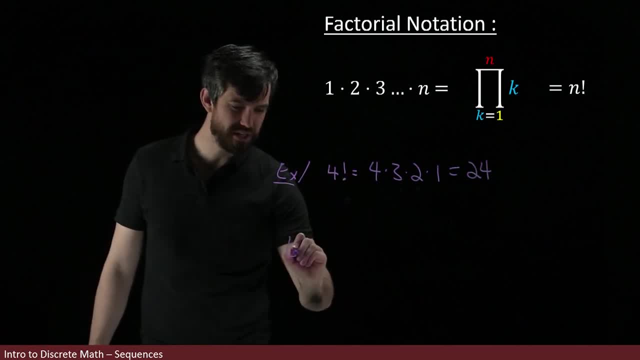 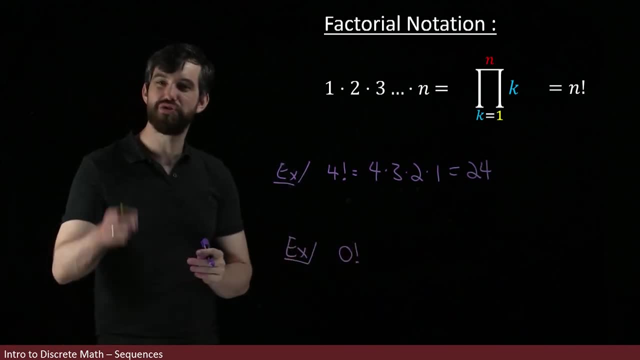 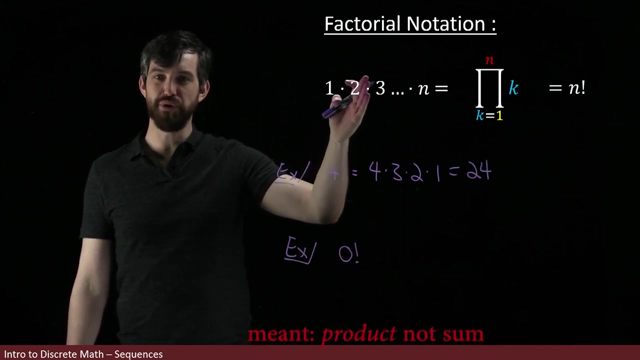 There's one sort of weird special case that I have to note, which is what happens if we take zero factorial And you might be tempted to think, oh, Trevor, it should be zero. But notice that in this particular sum you start at one, two. 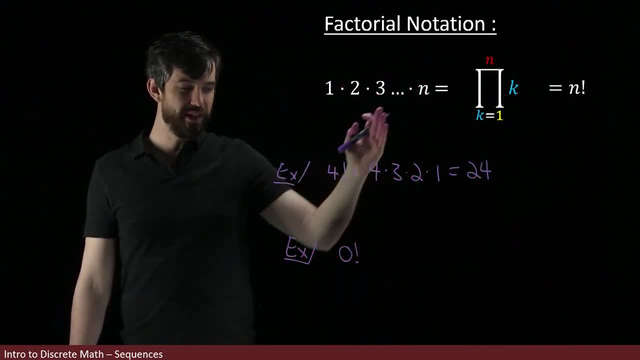 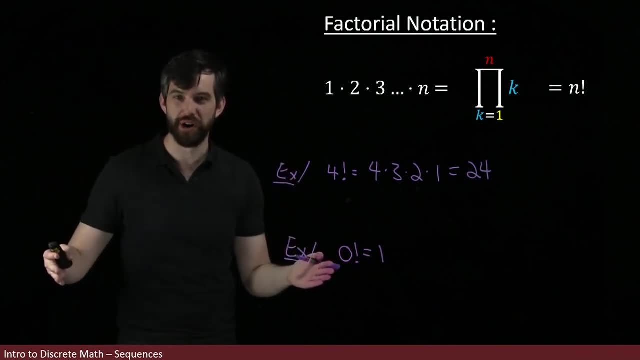 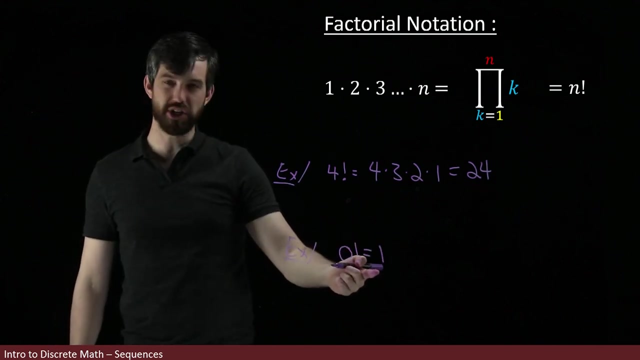 there is no spot for zero here. So this is actually defined a little differently. It's defined to be equal to one. So for a positive integer, n factorial is this thing. for the integer zero factorial is defined to be just zero. factorial is one. 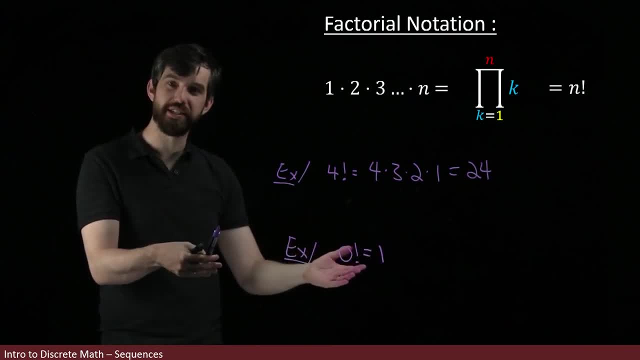 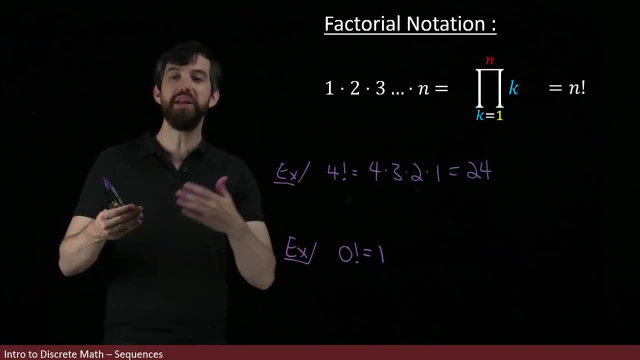 By the way, one of the reasons why we adopt this convention is that in the future, we're gonna connect this factorial, factorial notation to probabilities And we'll ask questions like: how many different ways are there that I can pull out some number from a bag that? 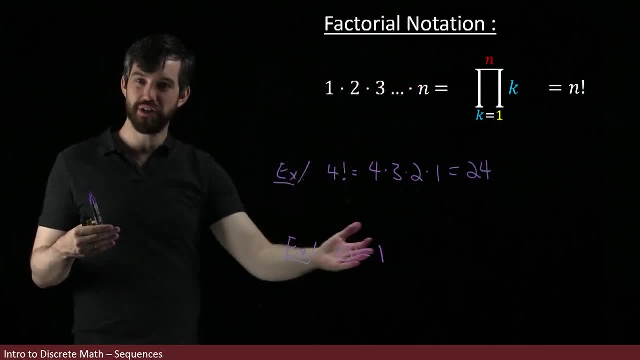 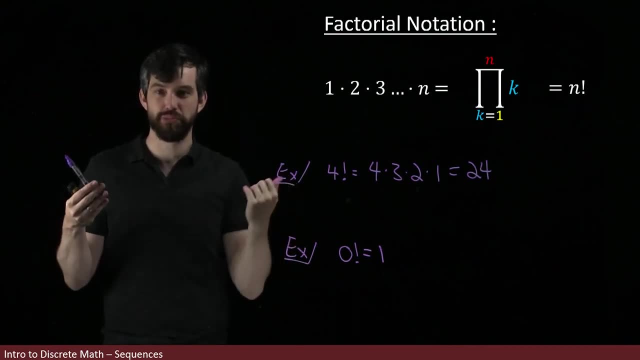 has all the numbers between 1 and n, And then the notion of 0 factorial is going to correspond to the idea that there is precisely one way where you can choose nothing. You just choose nothing. So there should be counted one way to choose nothing. 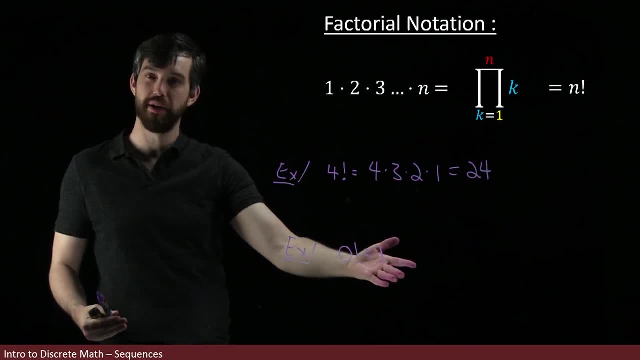 and therefore it's going to be defined in this kind of bizarre and strange way. But nonetheless, this is our factorial notation.